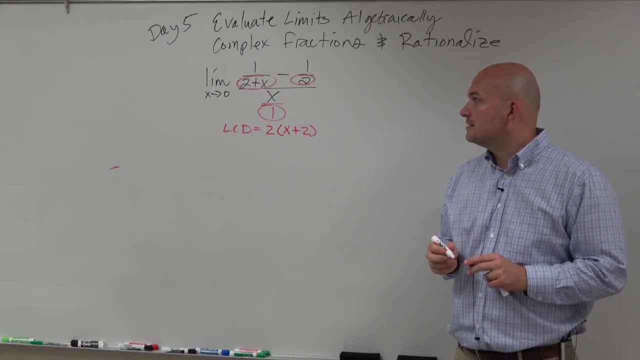 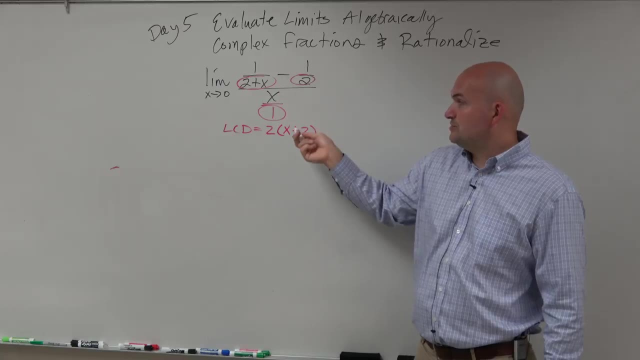 It doesn't really matter for that. OK, So that's going to be my common denominator, And I don't really need to write 1, because 1 obviously divides into it, But x plus 2 divides into that and 2 divides into that. 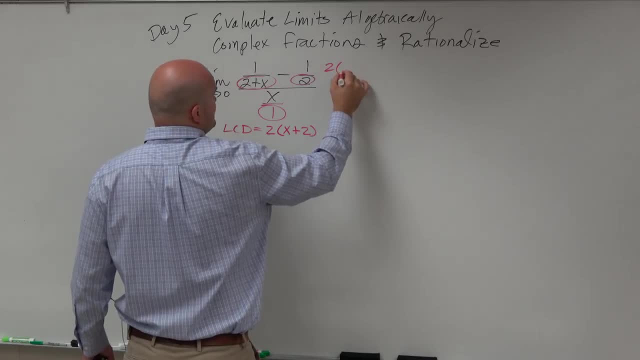 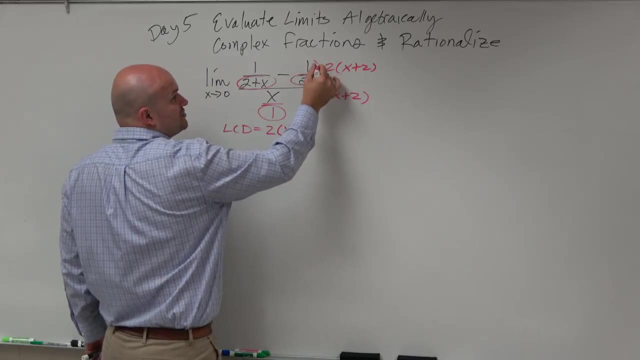 because they both. So now I'll multiply the top And the bottom by 2 times x plus 2.. Now watch, Oh, and you've got to remember, when you're multiplying this numerator, this complex fraction, you've got to remember you're multiplying. 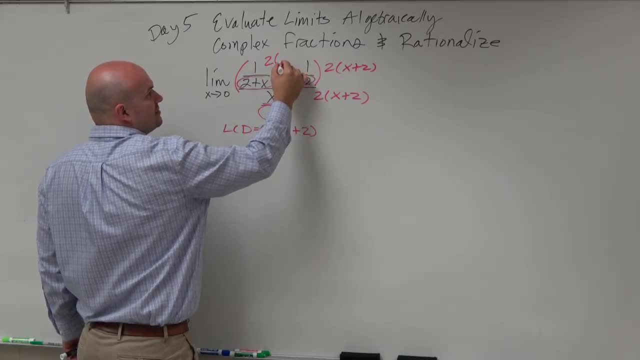 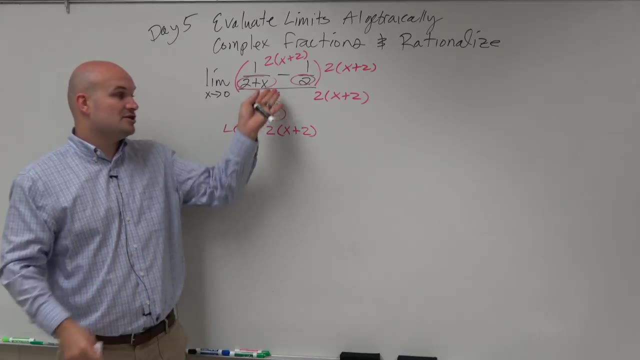 the top and the bottom. So a lot of times we'll just write it twice. You're multiplying basically every term When you're trying to get rid of your fractions. you're multiplying everything times your LCD. So what happens when I multiply 1 over 2 plus x times 2 times x plus 2?? 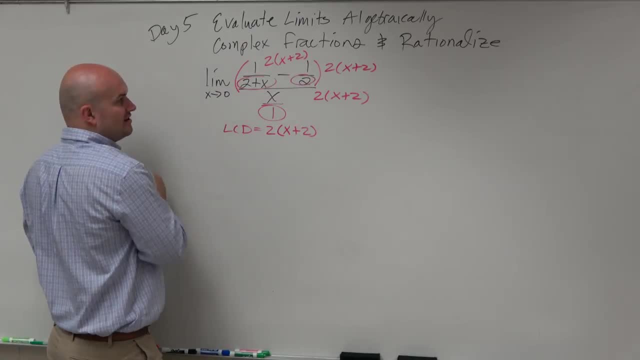 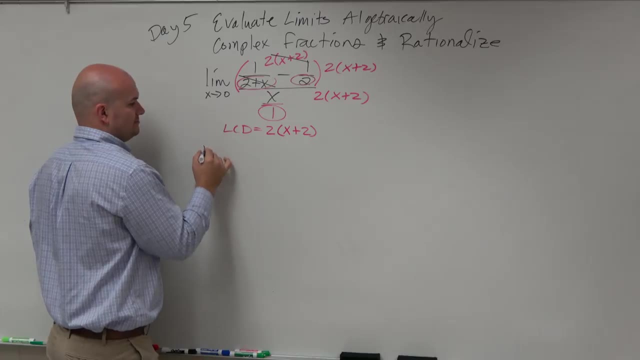 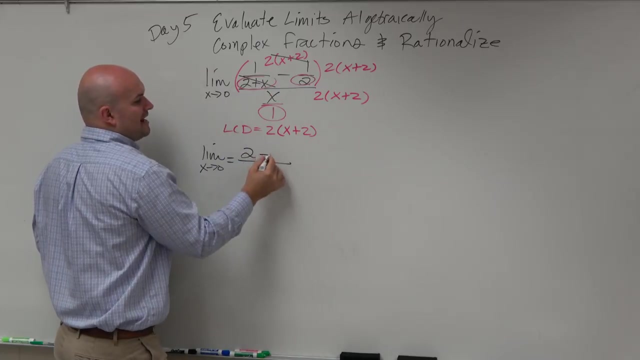 Well, again, these are the same. I'll just switch around. So, since this is the denominator that's in the numerator, they divide out to each other, right? So that's going to just leave me with 2. And then minus. 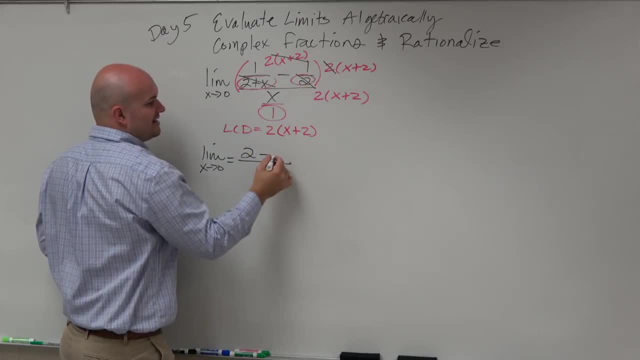 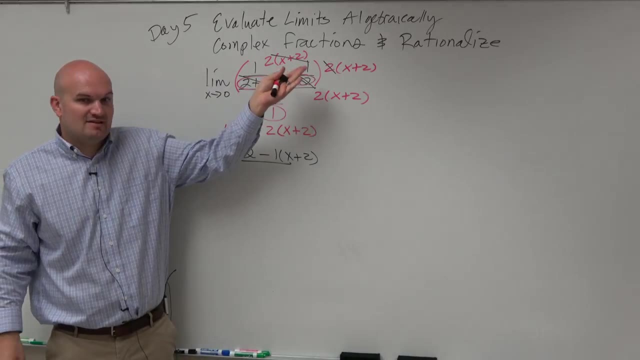 Now, here you can see that the 2's divide out. And again, guys, if you did this correctly, your denominators are always going to divide out, right, Because by choosing the LCD, you're choosing numbers. Right, You're choosing the numbers that your denominators divide into. 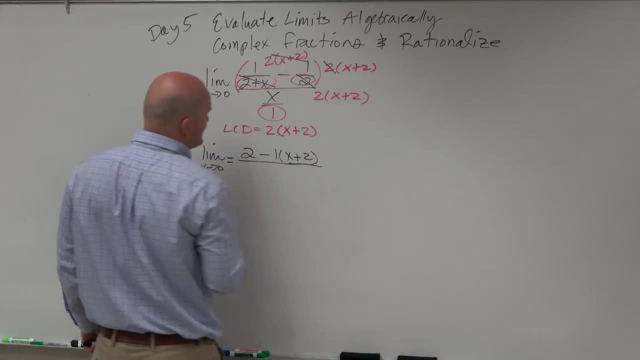 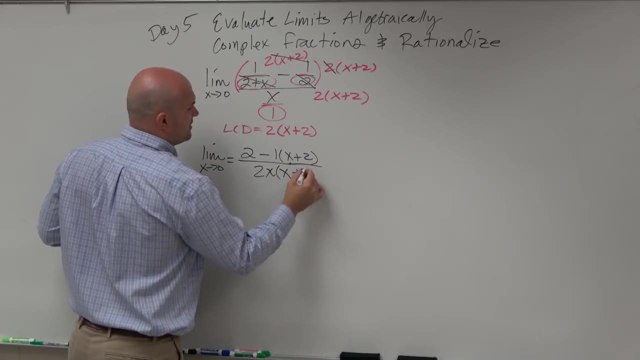 Right. So if you don't get rid of your fractions, then you obviously did something wrong. And then the denominator I'm going to have: 2 times x, times x plus 2.. Now I would recommend leaving it just like that, not doing anything else, not simplifying your denominator. 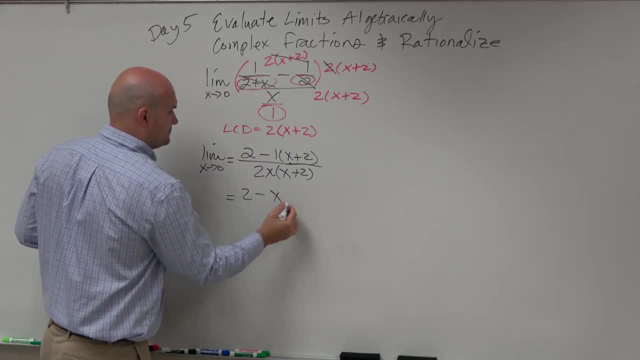 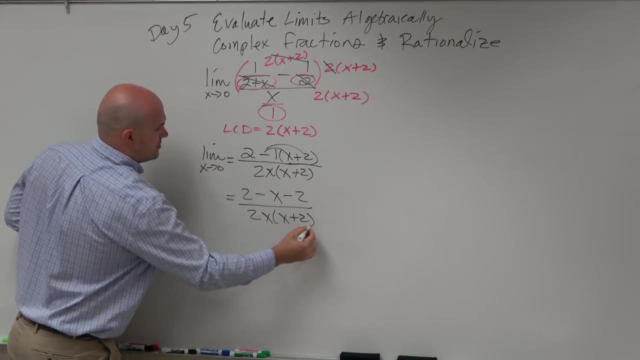 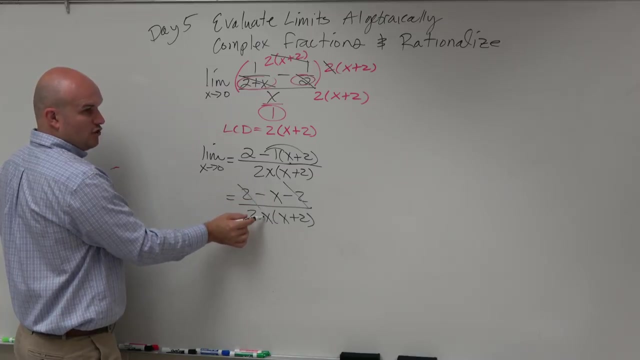 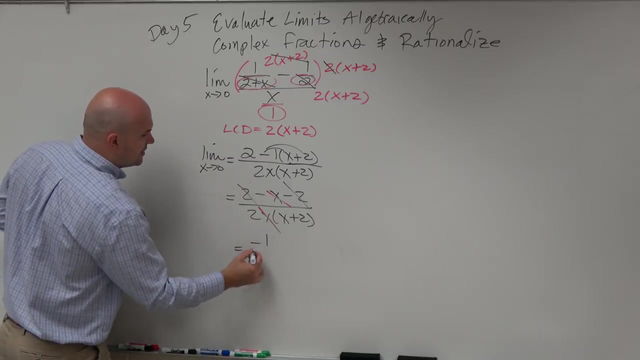 Because my numerator apply to strator property. you guys can see here now the 2's subtract out And then we're left with a negative x over x. Those also divide out And therefore we're left with a negative 1 over 2 times x plus 2.. 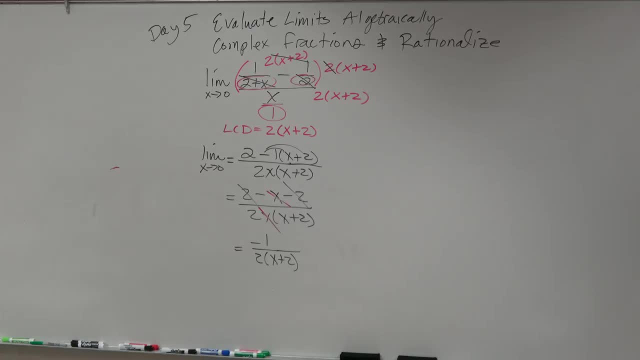 Now, after simplifying this, now can we directly substitute. Right Now can we directly substitute. Yeah, now it's perfect, right? We just had to simplify this a little bit. So, if I, as x, approaches 0, so we're just.